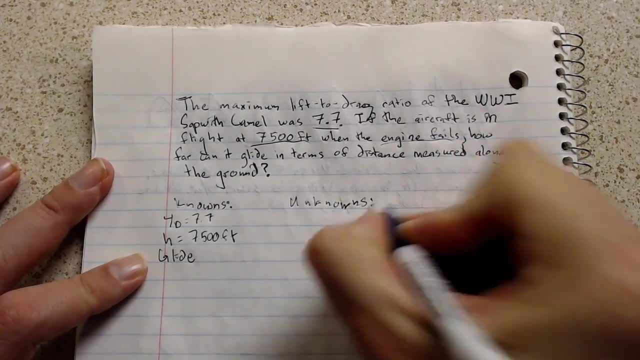 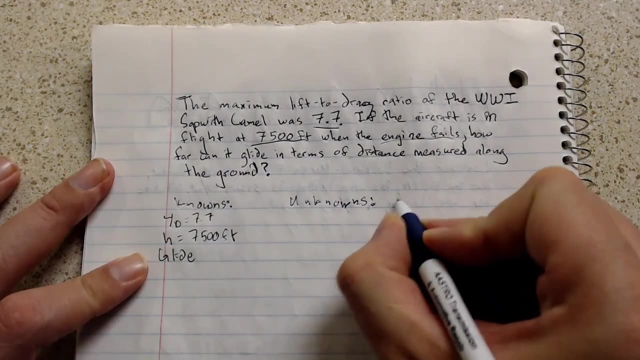 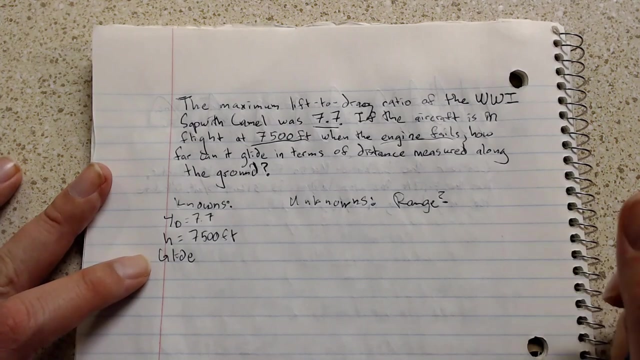 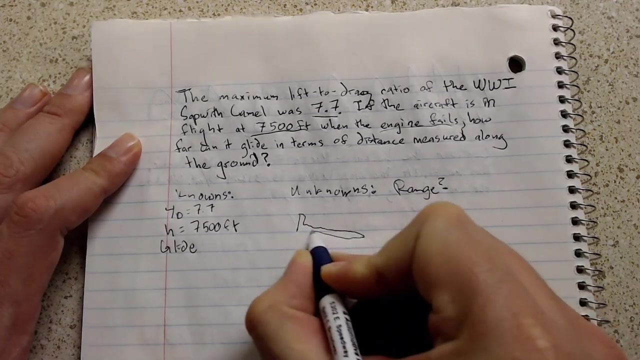 Our unknown would be the distance measured along the ground that it can go. We call this the aircraft's range. What is the aircraft's range? Let's go ahead and take a look at what this airplane will look like and the forces it will see in flight. I got a very poor drawing. 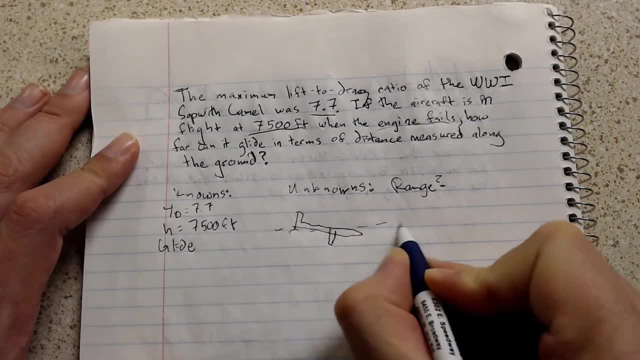 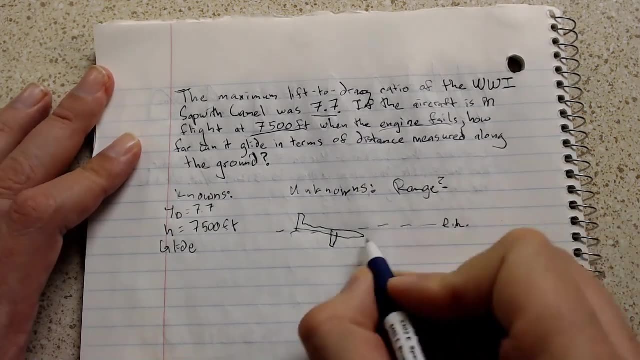 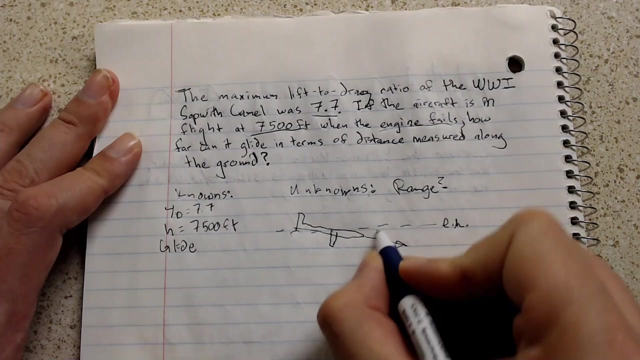 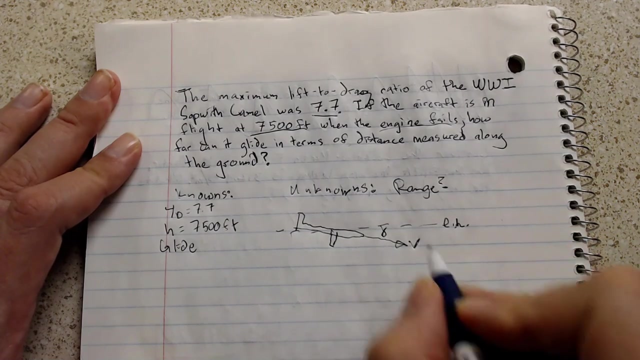 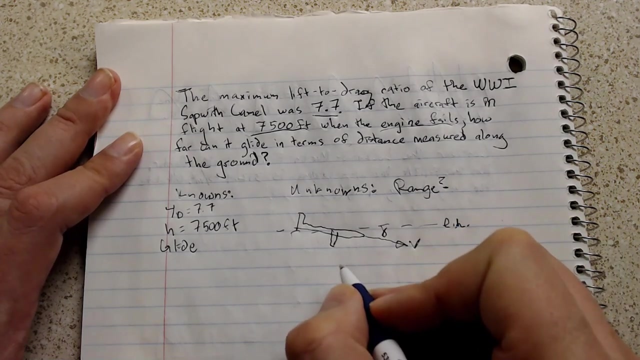 right here. Let's say: I have a local horizon. Go ahead and mark that local horizon Now, in a few seconds, I'm going to go ahead and mark that local horizon. So this is the actual travel path of the aircraft And, if we look at it, it's going to have three of the four. 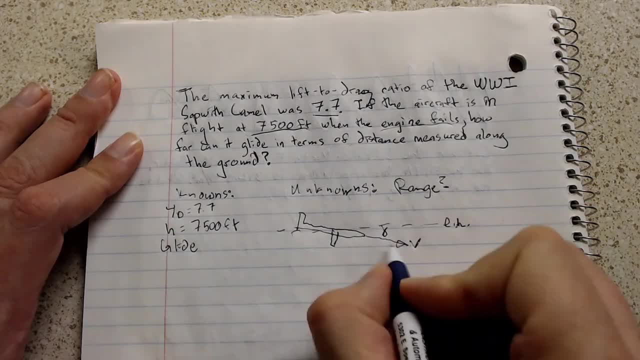 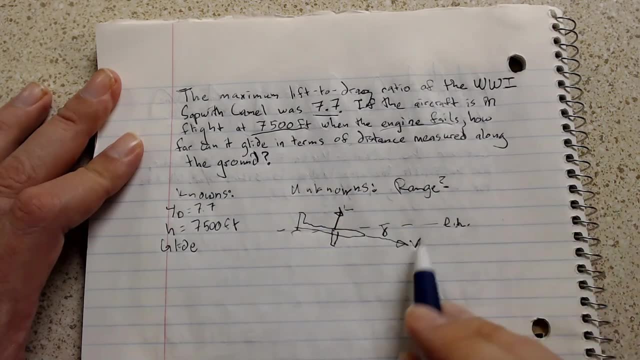 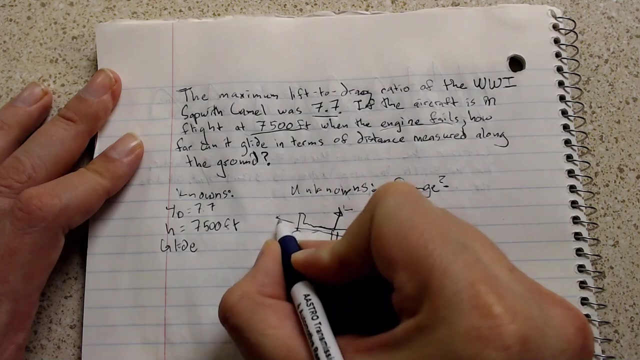 forces acting on it. It's not going to have any thrust because the engines are off. It's going to have a lift value, obviously perpendicular to this velocity. It's going to have a lift value. It's going to have a drag which I'm going to put back here. Oh, my pen, Come on pen. 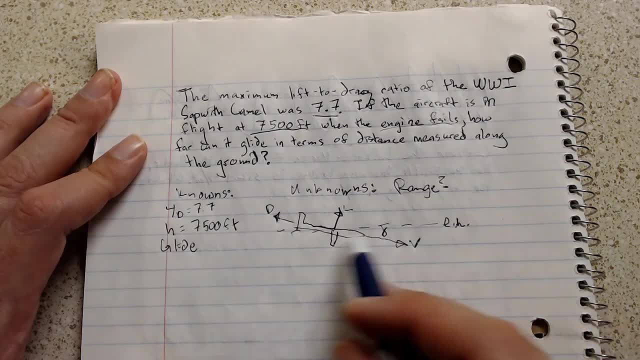 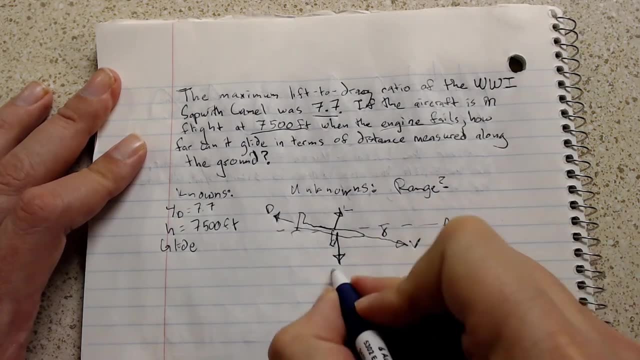 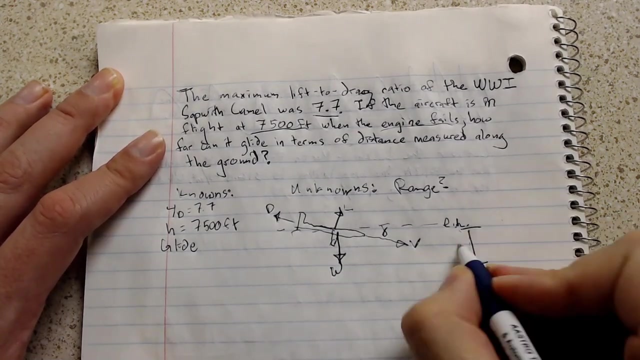 It's got a drag which is acting parallel but in the opposite direction to the velocity, And then it's going to have a weight which is acting straight down And of course we know the height that we're at and we're trying to figure out the range of the aircraft. 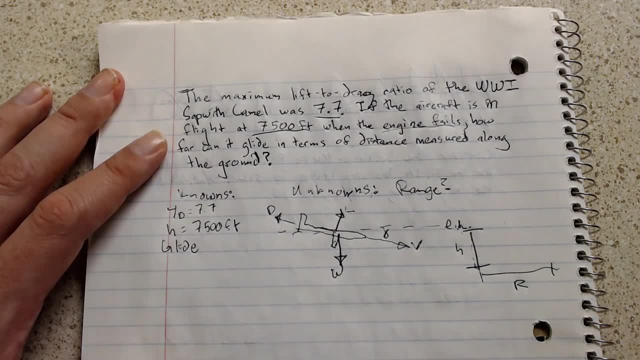 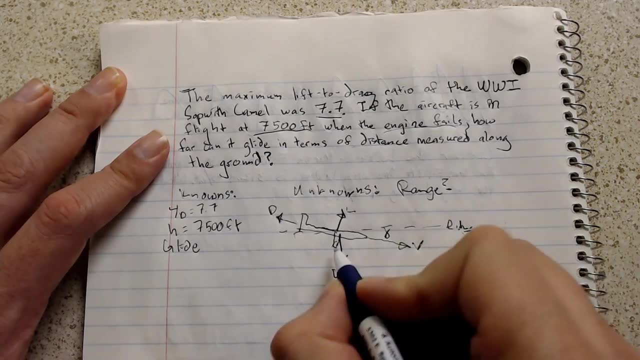 It's going to travel. Now, what we're going to do is we're going to take this weight value here, this weight vector. It's got a direction, And what we're going to do is we're going to split it up into a weight component. 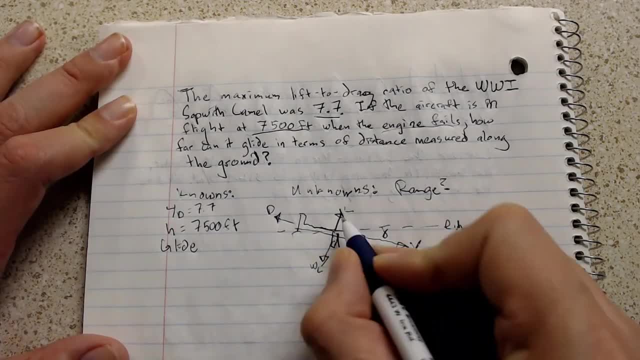 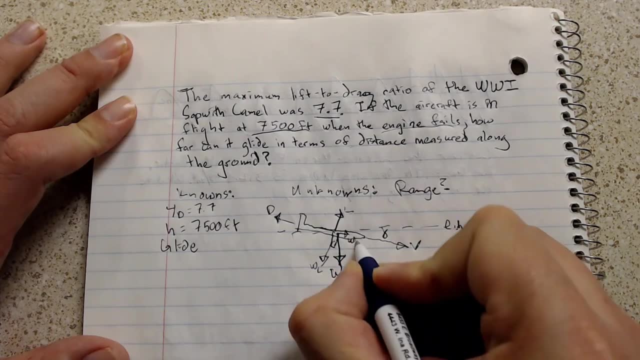 that acts along the lift vector, And then we can also have a weight component along the drag vector- Weight due to drag. Now, since we're in an equilibrium state where we're not accelerating, we're going to have a weight vector that acts along the lift vector, And then we can. 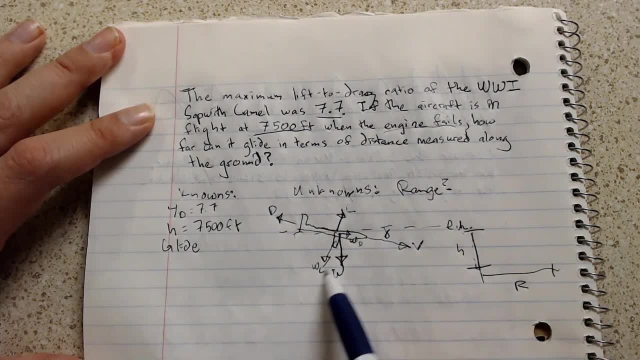 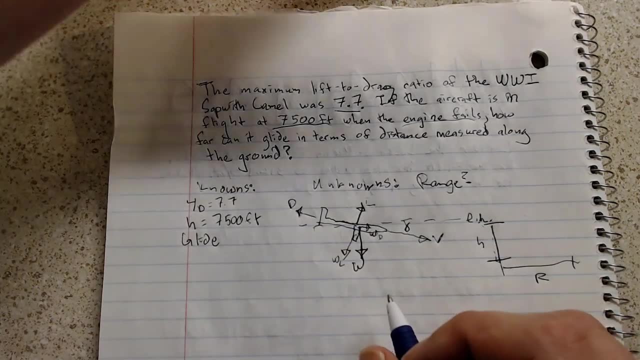 see that we're accelerating. The lift is going to have to equal this component of weight, and then the drag is going to also have to equal this component of weight. So if we write out those equations right here on the left, we'll get. 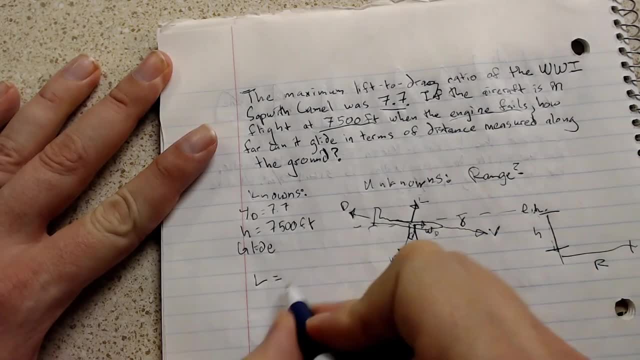 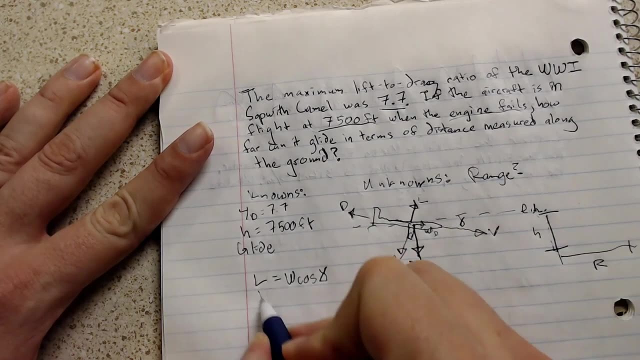 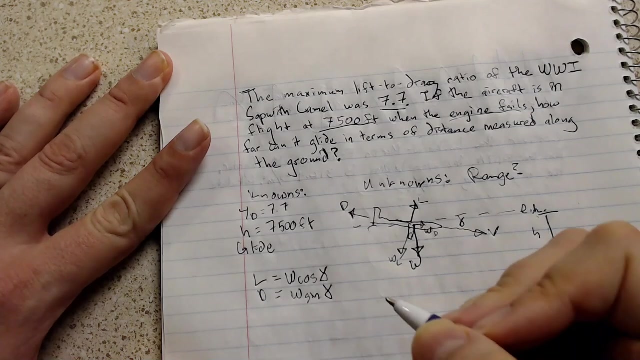 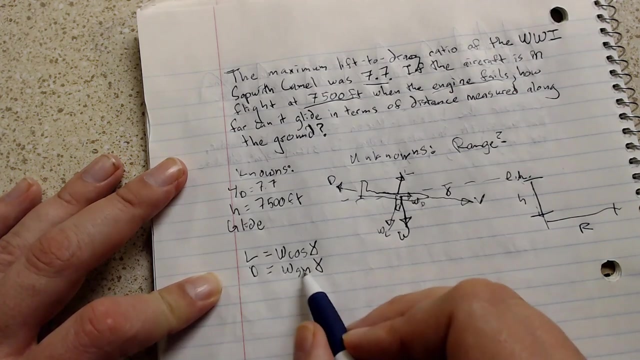 see, lift is equal to the weight times. the cosine of the flight angle- And then we'll also get drag- is equal to the weight times. the sine of the flight angle angle. Now, if you remember your trigonometry, tangent of an angle is the same as sine of an. 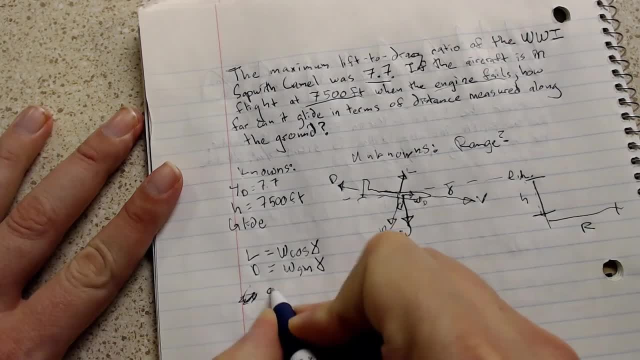 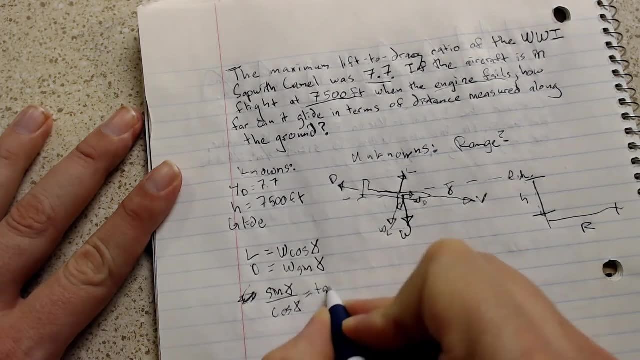 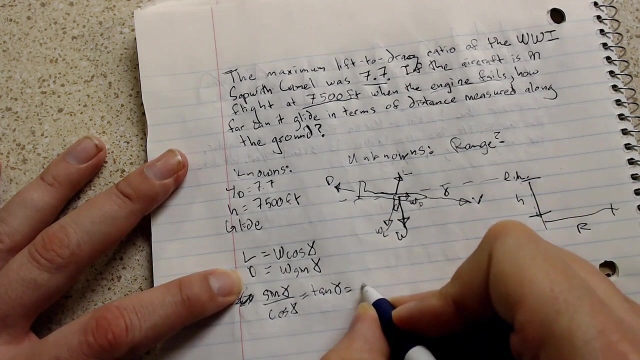 angle over cosine of an angle. If we flip these we can have sine of the flight path angle over cosine of the flight path angle equals tangent of the flight path angle And that is equal to the drag over lift or one over the lift to drag. 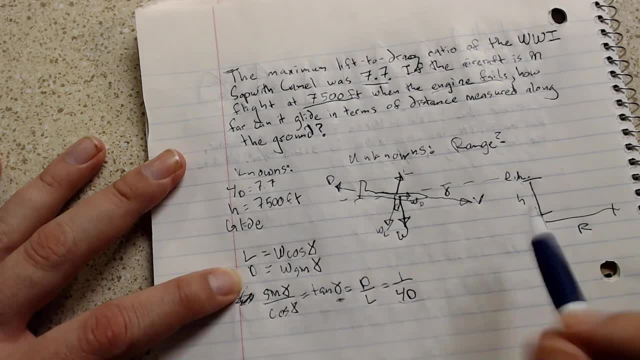 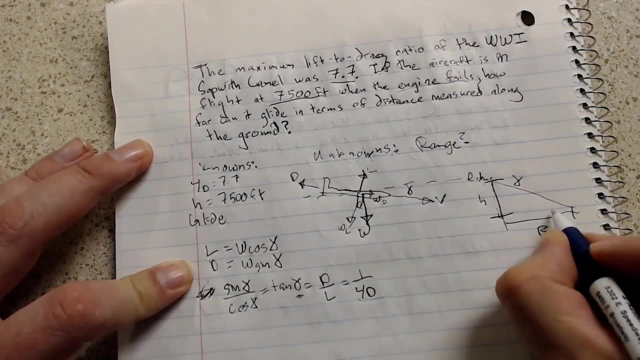 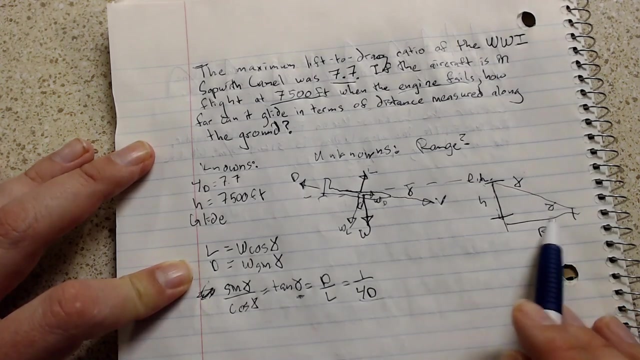 And we have that value. This will give us the flight path angle And with knowing the flight path angle over here, that's the same as this flight path angle over here. We can use some trigonometry to figure out what this range is. with this flight path angle and this height. 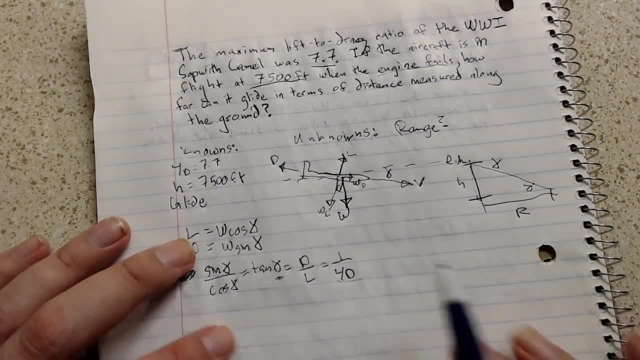 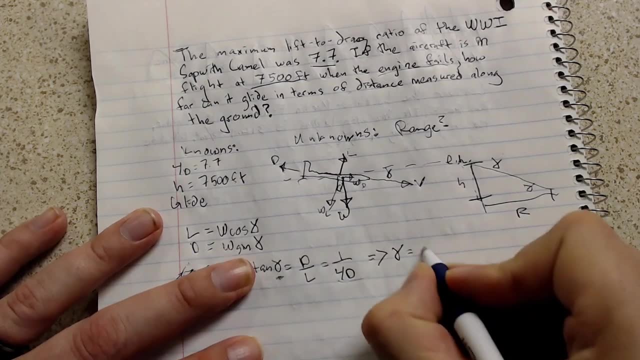 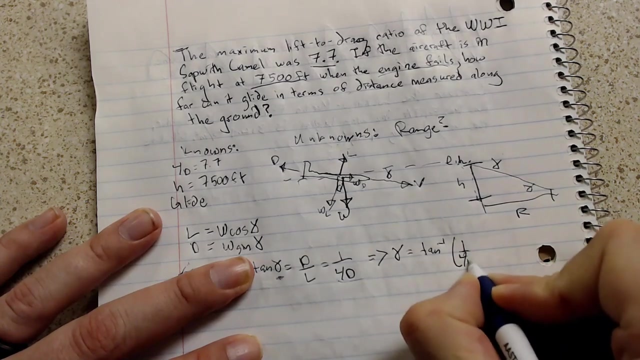 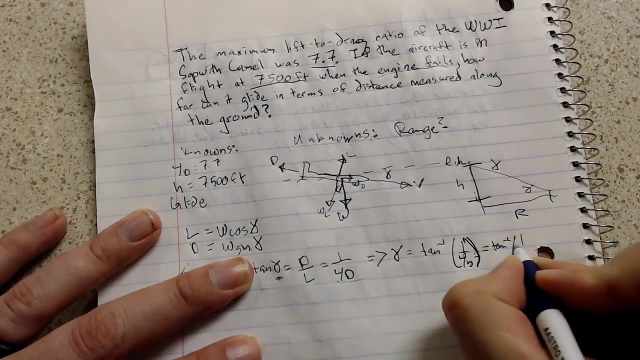 If that's what we're going to try and do, So rearranging this equation, the flight path angle is equal to tan inverse of one over lift to drag, which equals tan inverse of one over 7.7.. So we're going to do that here. So if we flip this ten over lift to drag, we can see that it is. 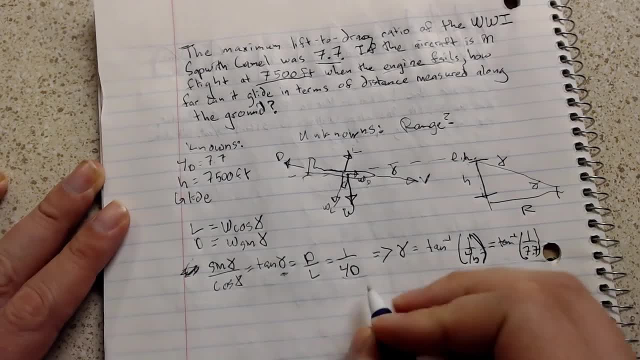 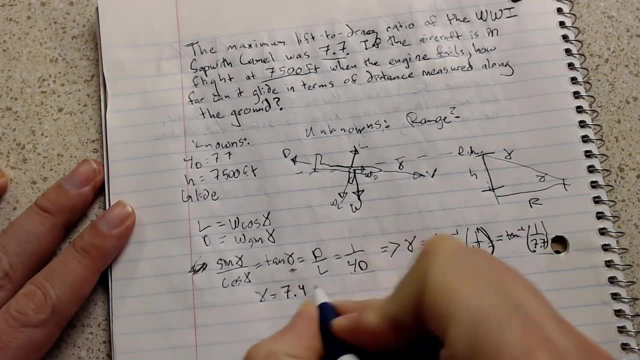 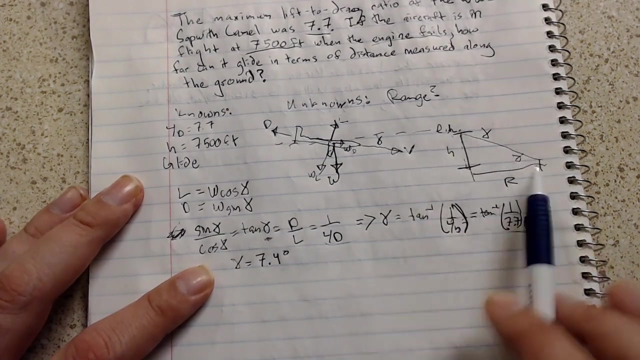 tangent of one over the lift to drag, which equals the tan inverse of one over seven point seven. plug this into your calculator. you're going to get a flight path angle of 7.4 degrees. Now, looking over here at the triangle that's made between the height, the range and the flight path, 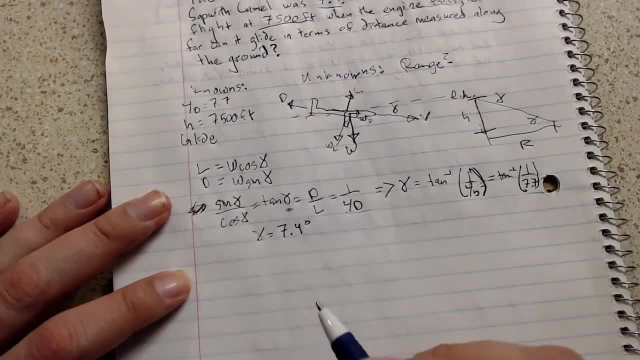 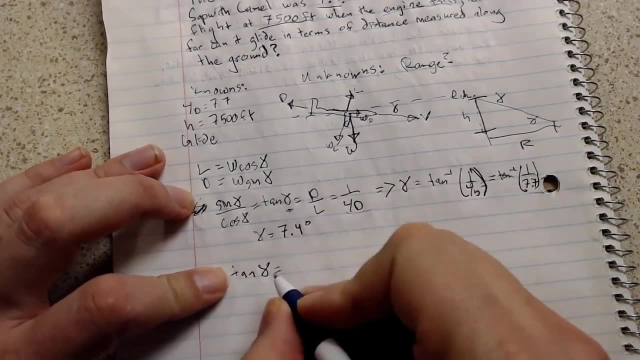 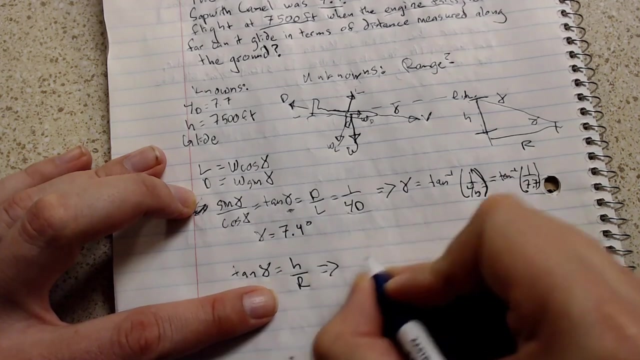 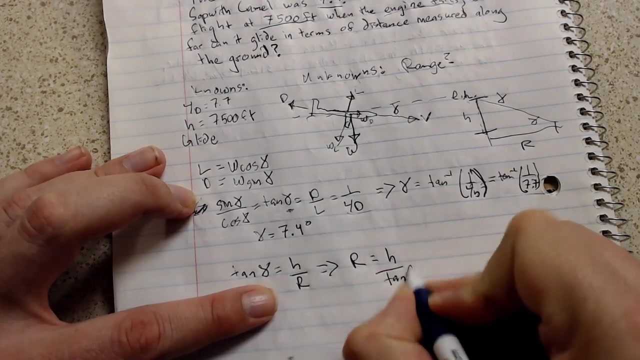 of the actual aircraft and using trigonometry, we know that tangent of the flight path angle is equal to the height over the range, And so what we can do is we can solve that for the range and range will equal the height divided by tangent of tangent of the flight path angle.